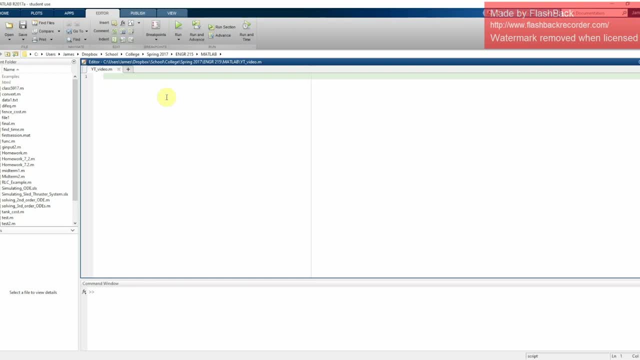 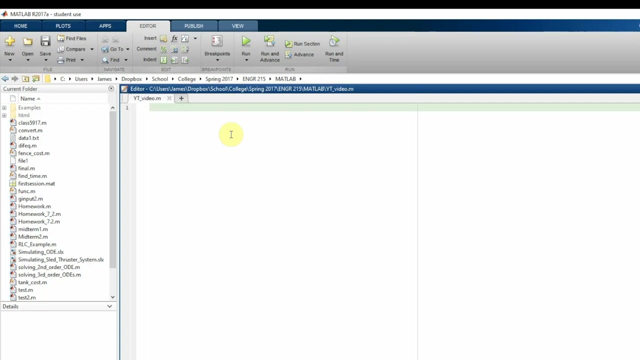 mathematical technique used to solve experiments and problems that are typically difficult or even impossible. They're used in fields of mathematics, physics and engineering. They're used for optimization and numerical integration. used to model complex systems with many degrees of freedom, such as fluids and certain materials. They can model kinetic models of gases. 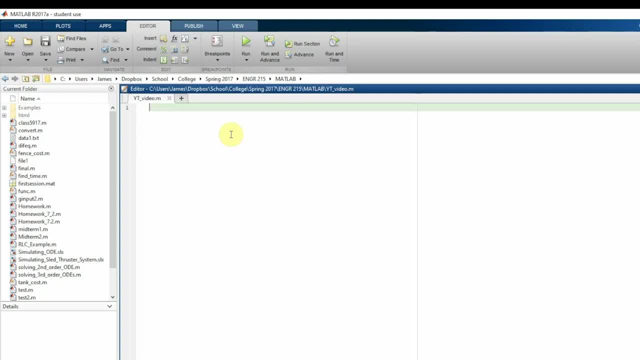 etc. They're used in engineering for microelectronics and fluid dynamics and signals and artificial intelligence. They're used in video games and video game AI. They're used in business and finance for estimating best and worst case and risk analysis. And yeah, so let's get into it. I'm going to show you how to write up some simple. 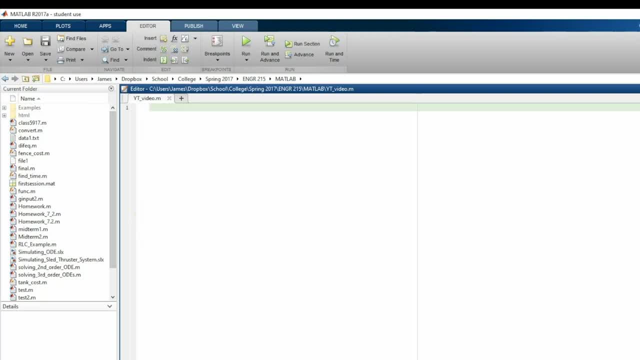 Monte Carlo simulations in MATLAB. Okay, so the first problem we're going to look at is we want to estimate the probability that five randomly dealt cards from a fair deck of 52 cards are all hearts. We're going to run the simulation a hundred thousand times and we're going to compare it to the theoretical probability. 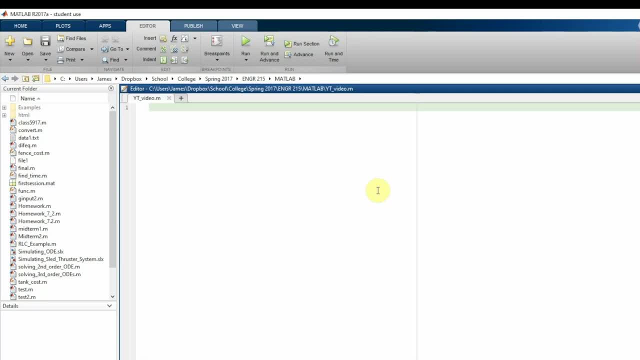 So the theoretical probability of drawing a hand of five hearts is given as 0.0049116.. And we want to use a Monte Carlo simulation, run it a hundred thousand times and see how close we can get to this theoretical probability. So the first step that I'm going to do in the simulation is create a variable. 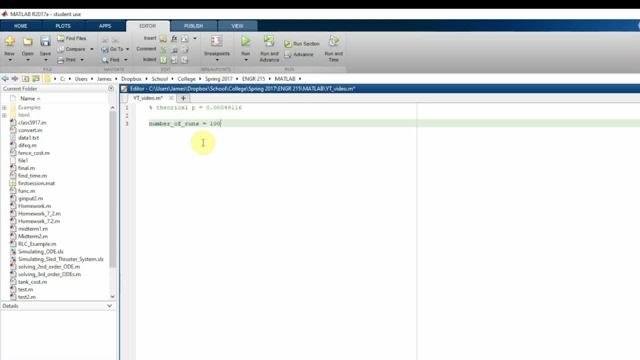 that will say how many times we're going to run the simulation. So it's called number of runs and I'm just going to set it equal to a hundred thousand because I want to run the simulation a hundred thousand times. This just makes it easy for, say, when you want to increase the number of. 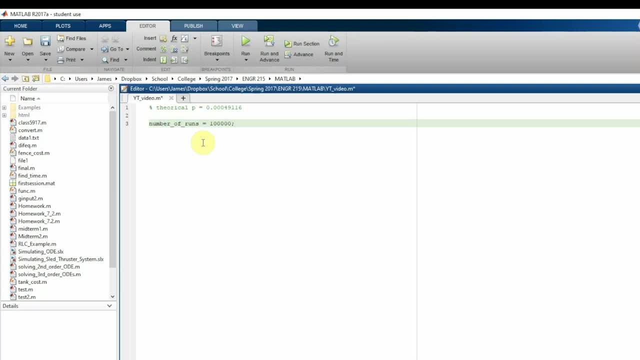 trials, or if you want to decrease it, then all you have to do is change this variable up here, because we're going to be using a lot of loops And we're going to be running loops and creating arrays of a hundred thousand elements. So instead 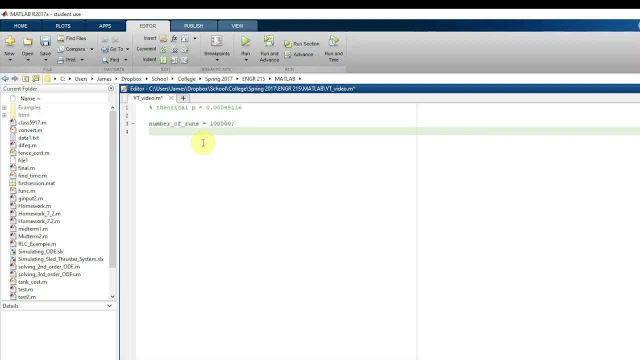 of changing all of them. we're just going to change one number up at the beginning, And then I'm going to create an array of 100,000 zeros. So it's going to be an array or a matrix of zeros. So I'm going to use zero function. It's going to create a one row. 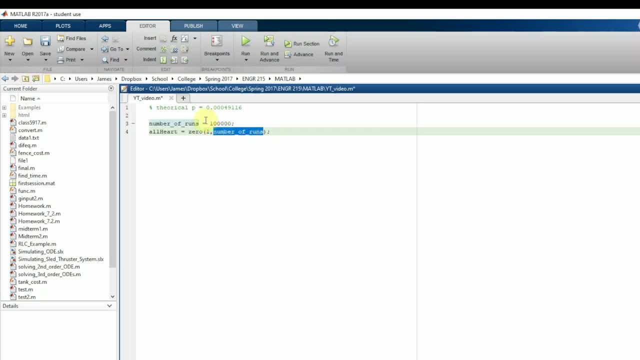 It's going to create a matrix, one row matrix, with number of runs, columns, So in this case it's a hundred thousand, And this is just going to keep track of how many times we've drawn a full hand of all hearts. So, for example, say, on the third trial of the simulation I get a full hand of hearts. Then I'm 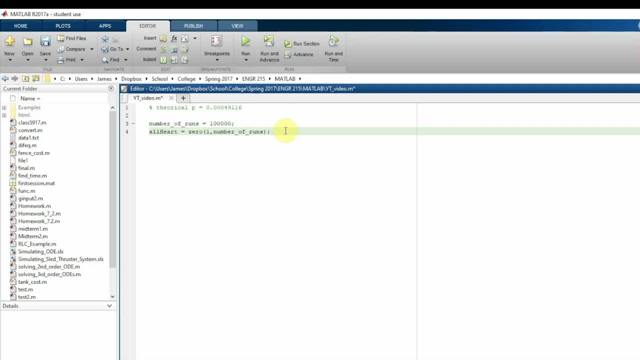 going to set the third column of this matrix equal to one. If I didn't get a whole hand of hearts, then I'm going to give it equal to zero And then we're going to add it up later and divide by the number of runs and that will give us our estimated probability. 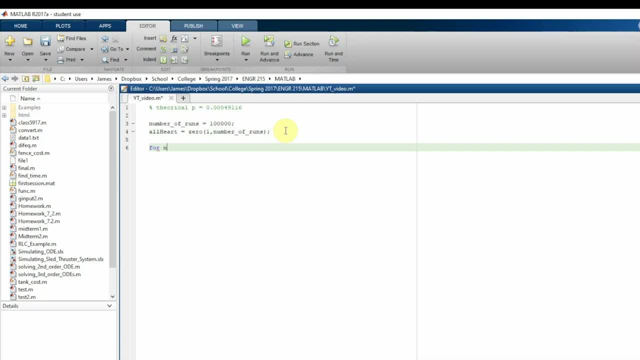 So we're going to want to run this 100,000 times. So we're going to create a for loop That's going to go from one to the number of runs, And then I'm going to create another variable called deck, which is going to use the randperm function in the built in matlab, which is going to 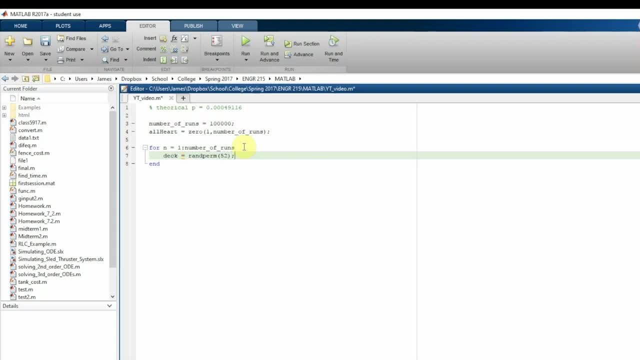 I'm going to put the number of runs 52, so this is going to. so deck is an array of 52 elements and random perm is going to fill in this array with a random permutation of the numbers 1 through 52.. so i'm also going to set another variable called number of cards drawn. 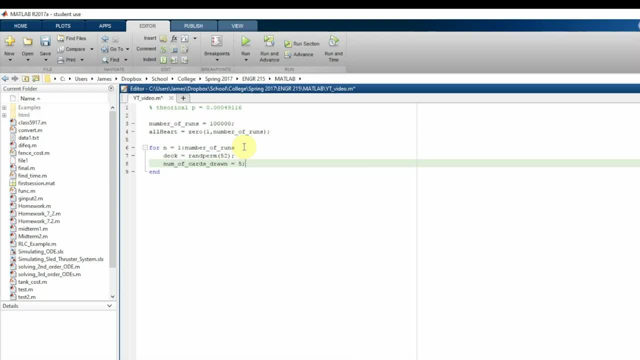 and i'm going to set this equal to five, so this just makes it easier if you want to run the simulation and you want to draw four cards, or you want to draw six cards, so instead of in our case, we're going to draw five, the top five cards. 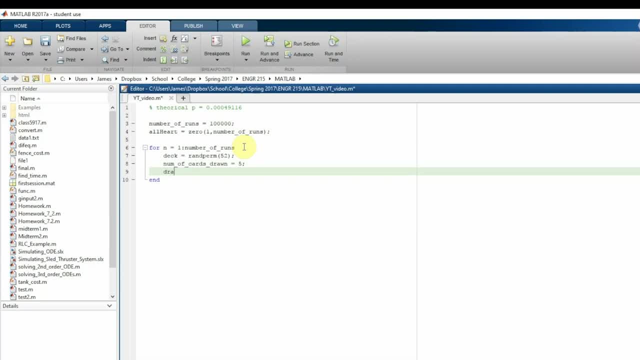 and then i'm going to create another variable this is going to. this is going to take the first five cards of our deck. it's going to draw the first card, the second card, the third card, all the way up until the number of cards drawn. in this case it's going to be five. so this is going to draw the top five cards of the deck. 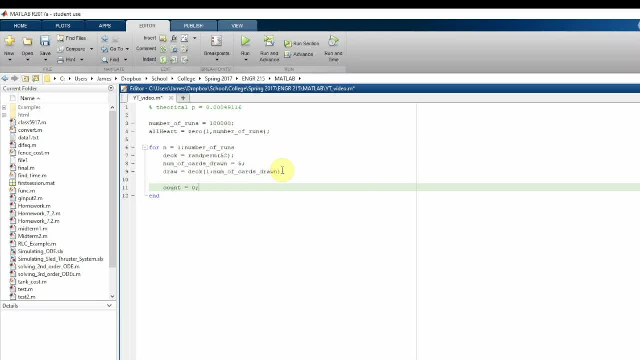 and then i'm going to have another variable called count, and this is going to count how many of the cards that were drawn are hearts, and we're going to initialize that as zero, and in another for loop for i equal to one number of cards drawn, and so we're going to say that we're going to try to get them all in the same row. 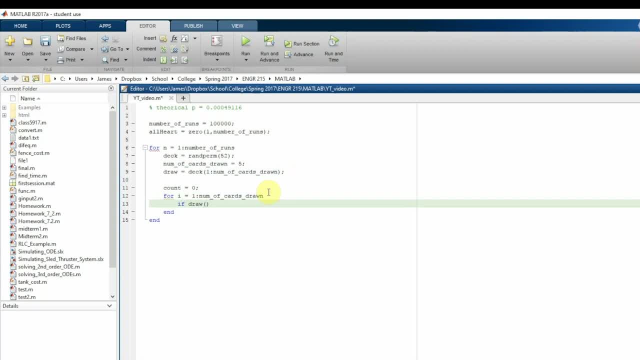 without shifting them between the top five and the bottom five. so very big problem. we need is at least this end point, and so that makes it easier for us to getting into the loop. so so we're going to select all the drawings and we're going to use the 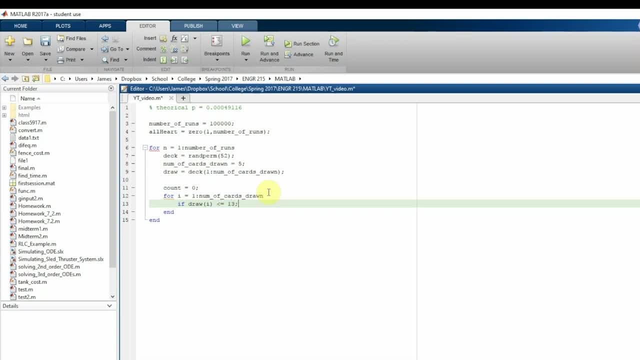 imens factoryama document. and we're going to say that if inside our hand of cards, that's what we call draw, if the index, i so from one to five, if that card is less than 13, then we're going to count, increment, count. the reason i'm using thirteen is because 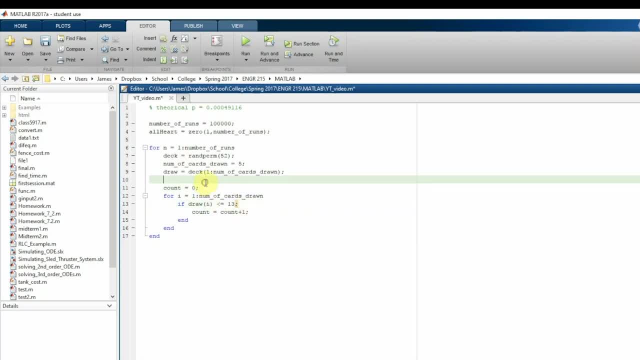 here, and so the idea is I have so in our deck, we have a random permutation of the numbers 1 through 52, and you have to have some way of signifying which cards go with which suit. so in this case, I only care about hearts. so either a card, 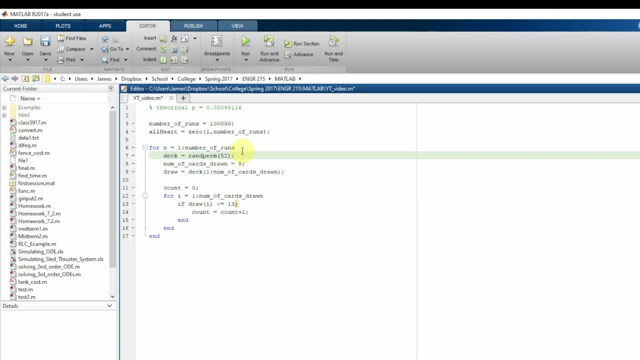 is a heart or it's not a heart, and so what I'm? so there's four suits in a deck. 52 divided by 4 is 13. so I'm saying that the first 13 numbers. so, from 1 to 13, these are all hearts, and from 14 to 52, these are all not hearts. so if we draw a 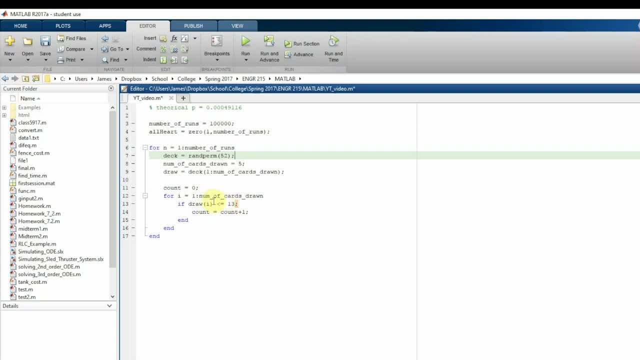 card you and it's less than or equal to 13, then we're going to increment our count and our count just says how many hearts in the draw in our hand that we have. okay, so this is going to count how many. this for loop is going to count how many. 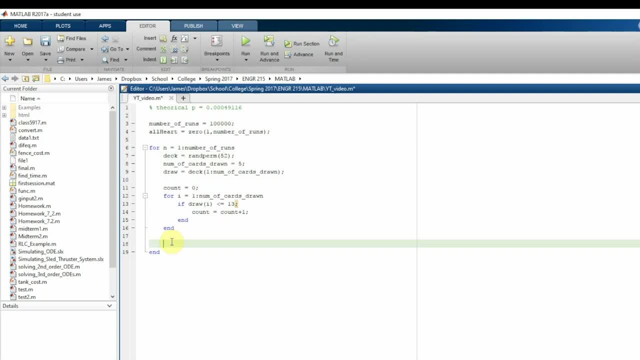 hearts we have in our hand, and then we're going to create another if statement, say, if count is equal to no more cards. so what this is gonna do is it's gonna see if we've drawn a full hand of hearts. so if count this variable up here, if it's equal to 5, then we're. 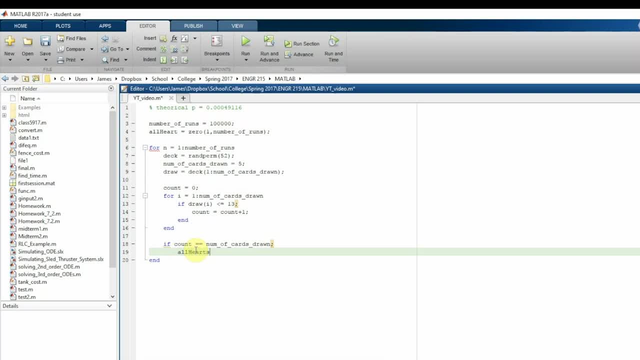 gonna set this, this huge array that we made earlier. so the element that corresponds to the entire array is equal to 5 and this is a very important element- the trial that we're in say we're in the first trial. if in our first trial we get 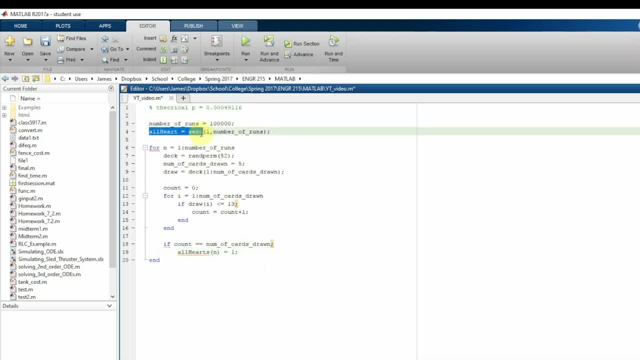 all hearts, then it's going to set the first element of this all heart array. it's going to be set to one and that means we got one full hand apart of hearts. else it's going to say all hearts is equal to zero, and so this is actually not. this else is not necessary, because 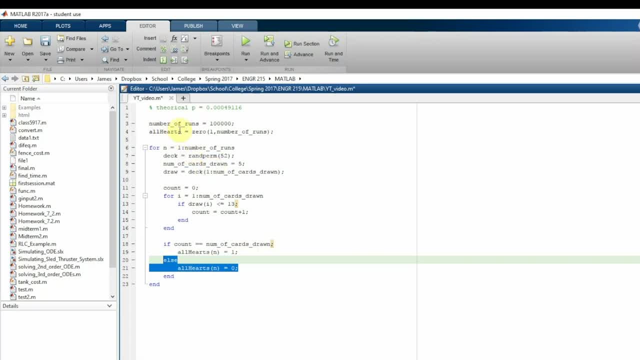 it's already. it's already zero in this case and we're just gonna set it to one if it's if we draw all hearts. but it's already zero in this case and we're just gonna set it to one if we draw all hearts, but. but I'm just going to keep it in there for simplicity.